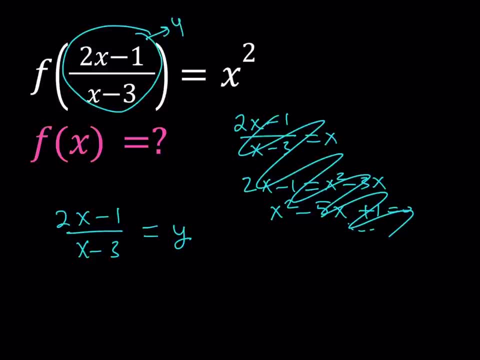 I'm setting this whole thing equal to y because I want to be able to get f of x, but for the time being I'm going to use another variable until I get a nice expression, and then I can replace y with anything I want. Okay, we'll talk about that a little later. So now what happens on the right? 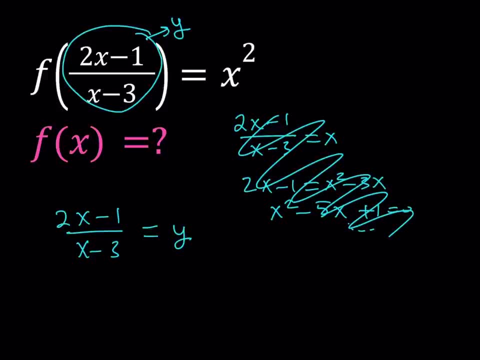 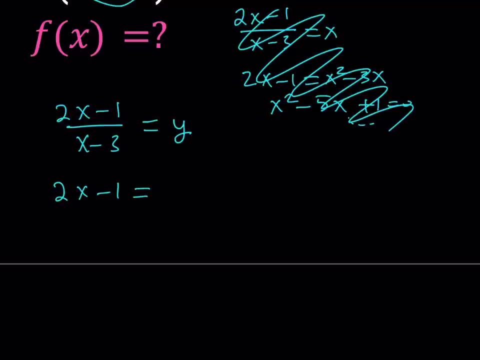 hand side. Since I have x squared, I have to be able to replace x with some signal. So let's go ahead and solve this in terms of x Cross multiply. And then I want to solve for x. So I want to bring the 3y over here and the 2x here. In other words, 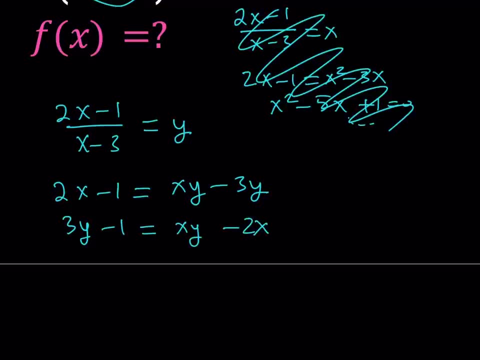 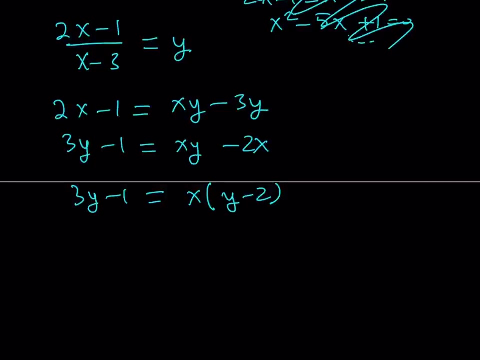 I'm subtracting 2x from both sides and I'm adding 3y to both sides. Now we can factor out x and from here I'm able to solve for x if we divide both sides by y minus 2.. Of course I know we have. 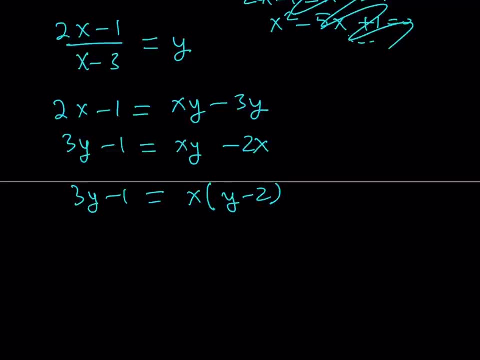 to talk about the domain and range. but as long as these values are appropriate, this function is going to be defined. So basically, we're talking about a function where it's defined. So from here let's isolate x. It's going to give me 3y minus 1 over y minus 2.. So our original expression: if 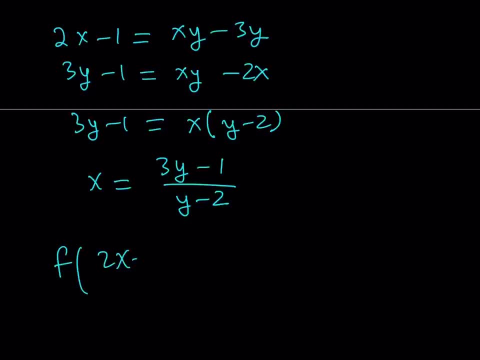 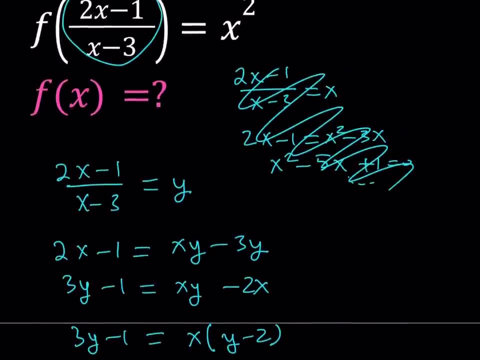 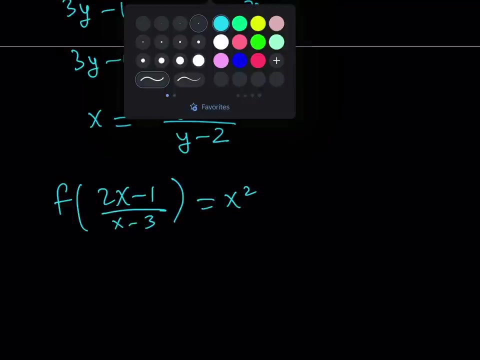 you remember it was f of 2x minus 1 over. x minus 3 is equal to x squared. So now we have to find the f of x here. Now I noticed that by replacing this with y, I'm basically replacing x with this. So 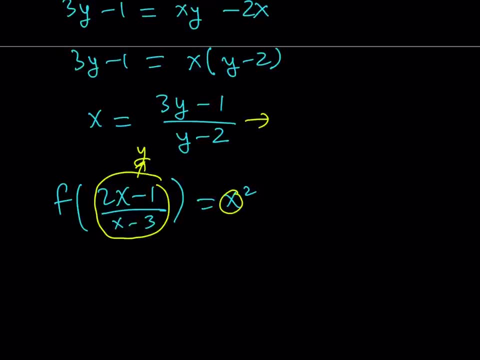 let's go ahead and replace x with this on the right hand side. So this is going to be: f of y is equal to x squared, but x will be replaced with 3y minus 1 over y minus 2.. And of course, I need to. 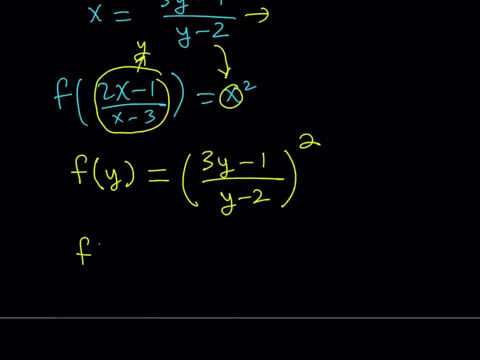 square that. If you square this expression, you're going to be getting f of y is equal to 9y squared minus 6y plus 1, over y squared minus 4y plus 4.. Now, I didn't get f of x, I got f of y, but that's. 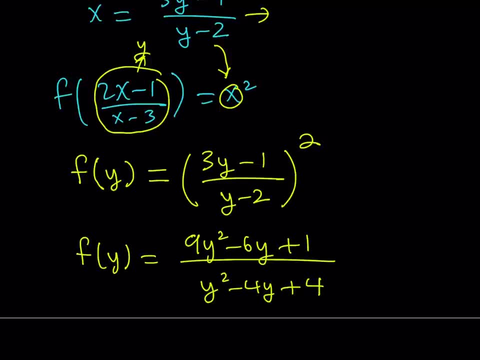 okay, I think this was the confusing part- like how come you replace x plus squares of x plus 1 with t and then you go ahead and replace t with x? How is that possible? Well, those x's are not the same, because I can use any variable I want right In a function. you can replace this y with, you know, t. 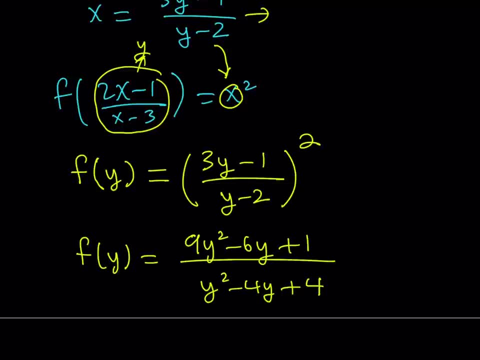 you can replace y with z, anything you want. You can even replace y with x- cubed. Of course there are some limitations, you know. we need to consider the domain and so on and so forth. but as long as they're satisfied, you have the freedom. So that's basically what I did for the other video: replace. 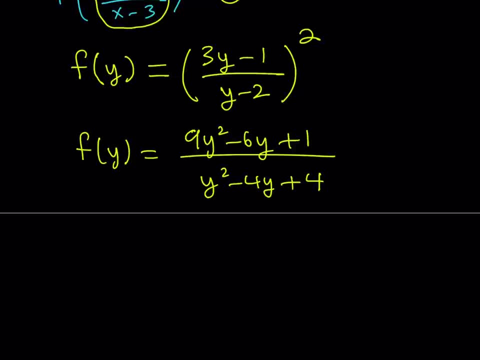 the variable with what I wanted, And we're going to do the same thing here. I want to get f of x, so my function in terms of x, but I have it in terms of y. but no worries, we can just go ahead and replace y with x on both sides. So here's the idea, as long as you're doing it on both sides. 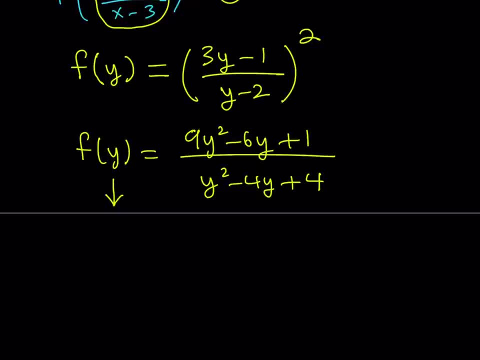 you're good. Okay, so let's go ahead and replace y with x, and that's going to give us f of x equals 9x squared minus 6x plus 1 divided by x squared minus 4x plus 4.. Of course, we have to consider the domain here. x cannot equal 2, you know, so on and so forth. 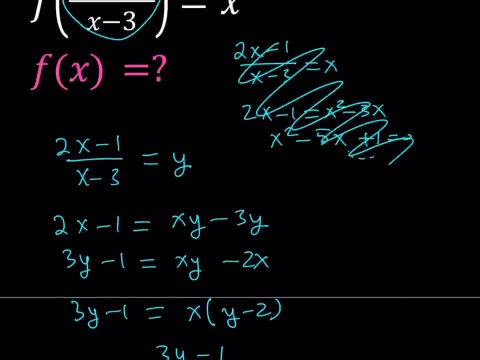 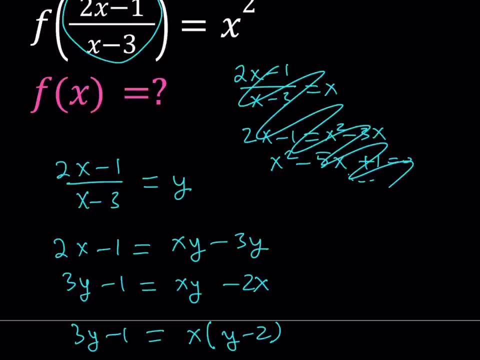 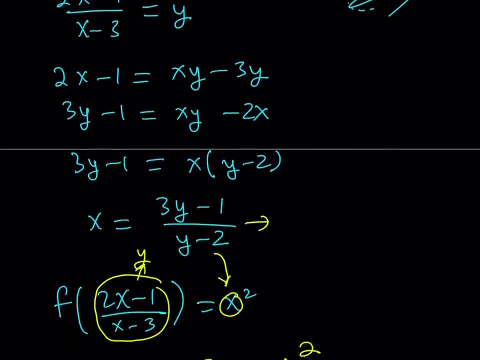 For the original problem. if you think about it, the domain is going to limit, x equals 3, is not defined, so on and so forth. So those values are going to work together. but you just have to consider those cases. Now I want to say another thing here. for this functional equation We got 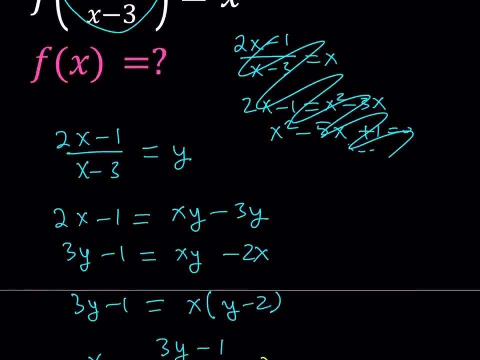 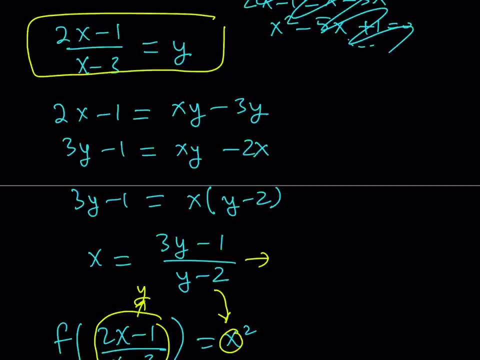 the answer, but I just want to emphasize one thing here which I believe is important. So what did we do by setting this expression equal to y and solving for x? Well, actually we found the inverse of this function, because this gives us if f of something equals y. 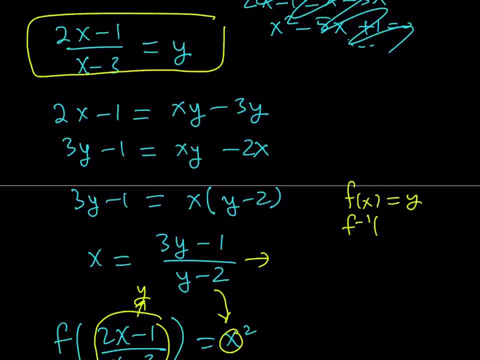 and you replace x and y, you're basically saying that f- inverse of y, is equal to x. by switching these around right? So this is kind of like the inverse of our function, but expressed in a different variable. So if you already knew that this function here it's a rational function and